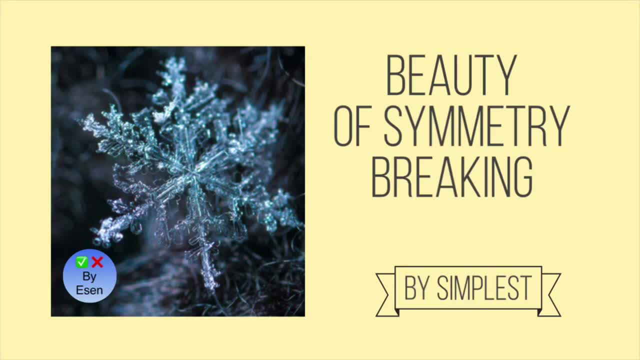 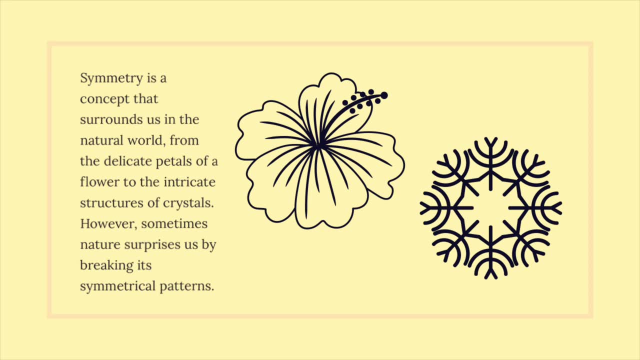 Beauty of Symmetry: Breaking By Simplest. Symmetry is a concept that surrounds us in the natural world, from the delicate petals of a flower to the intricate structures of crystals. However, sometimes nature surprises us by breaking its symmetrical patterns. Let's assume there is perfectly symmetrical hill with symmetrical two. 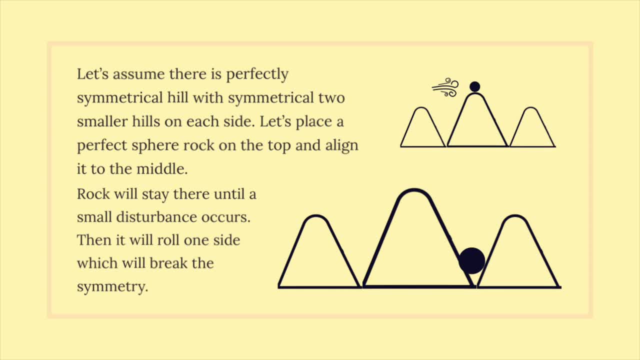 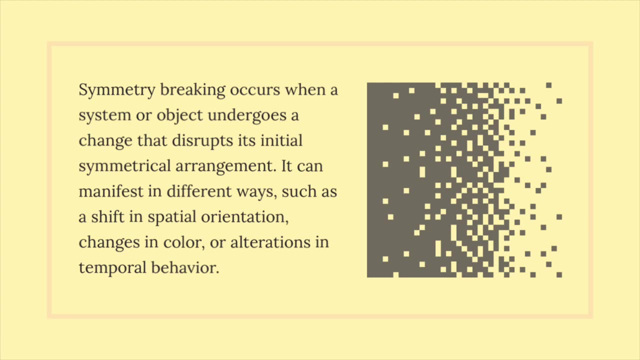 smaller hills on each side. Let's place a perfect sphere rock on the top and align it to the middle Rock will stay there until a small disturbance occurs. Then it will roll one side, which will break the symmetry. Symmetry breaking occurs when a system or object undergoes a change that disrupts its initial. 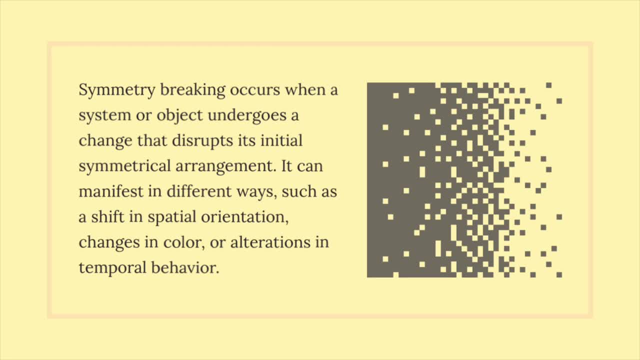 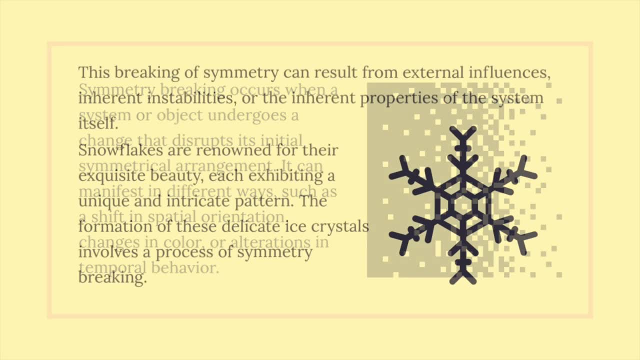 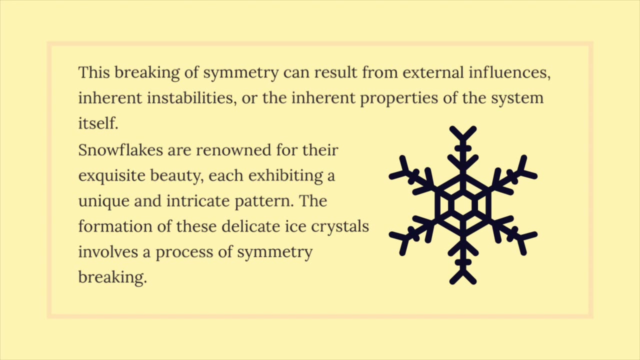 symmetrical arrangement. It can manifest in different ways, such as a shift in spatial orientation, changes in color or alterations in temporal behavior. This breaking of symmetry can result from external influences, inherent instability or the inherent properties of the system itself. Snowflakes are renowned for their exquisite beauty. 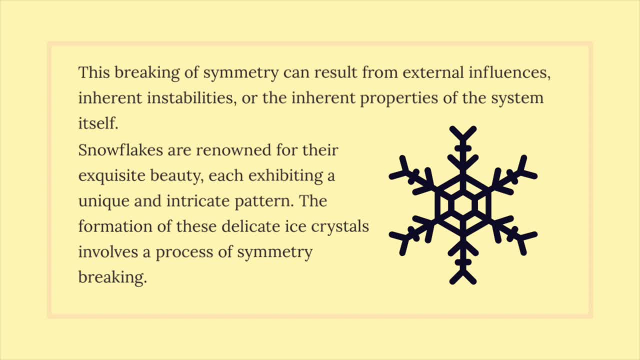 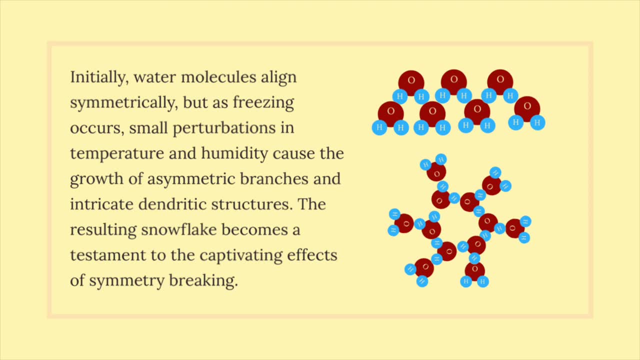 each exhibiting a unique and intricate pattern. The formation of these delicate ice crystals involves a process of symmetry breaking. Initially, water molecules align symmetrically, but as freezing occurs, small perturbations in temperature and humidity cause the growth of asymmetric branches and intricate dendritic structures. The resulting snowflake becomes a testament to the captivating 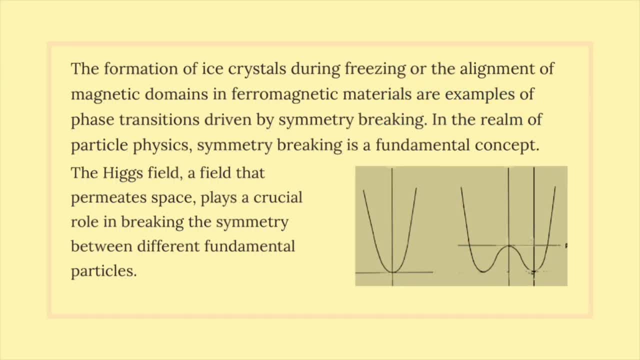 effects of symmetry breaking. The formation of ice crystals during freezing or the alignment of magnetic domains in ferromagnetic materials are examples of phase transitions driven by symmetry breaking. In the realm of particle physics, symmetry breaking is a fundamental concept, The Higgs field, a field that permeates space. 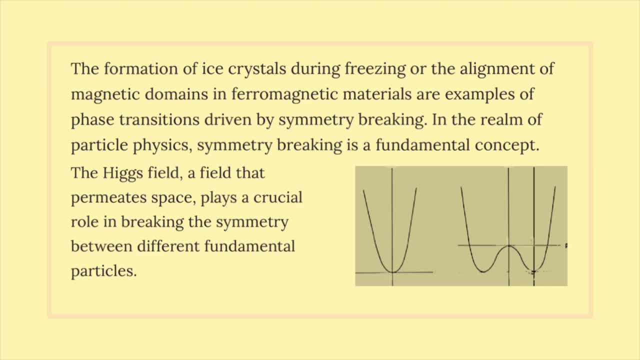 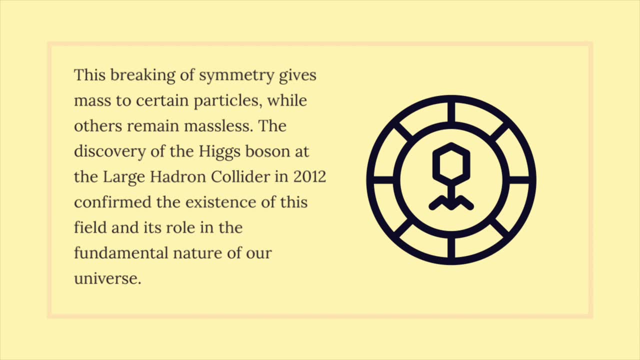 plays a crucial role in breaking the symmetry between different fundamental particles. This breaking of symmetry gives mass to certain particles, while others remain massless. The discovery of the early phytoplankton is a fundamental aspect of spatial science. of the Higgs boson at the Large Hadron Collider in 2012 confirmed the existence of this field. 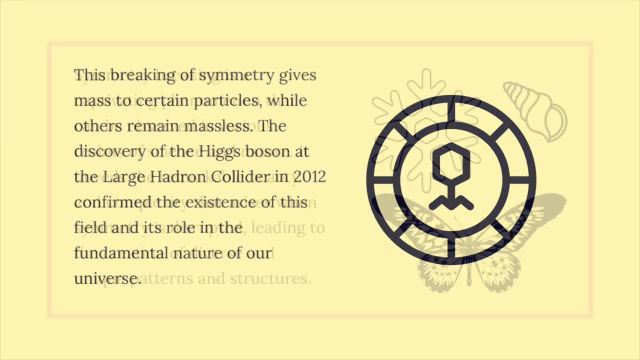 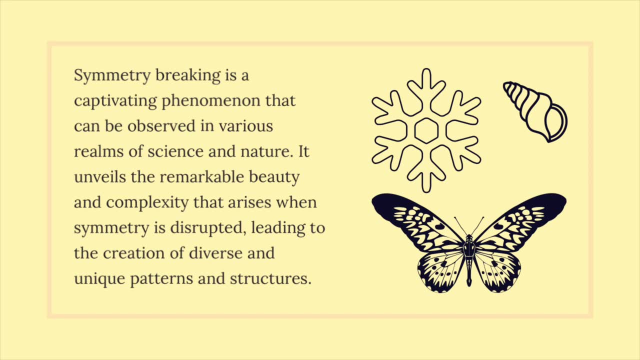 and its role in the fundamental nature of our universe. Symmetry breaking is a captivating phenomenon that can be observed in various realms of science and nature. It unveils the remarkable beauty and complexity that arises when symmetry is disrupted, leading to the creation of diverse and unique patterns and structures.